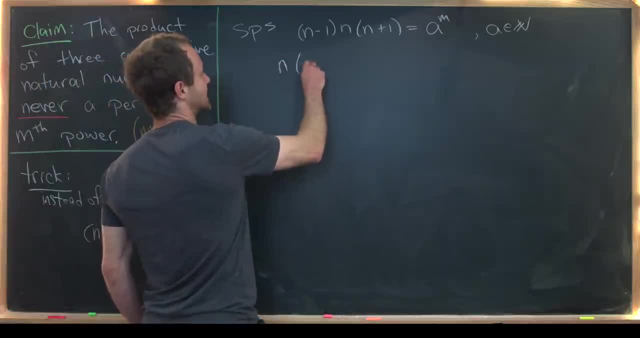 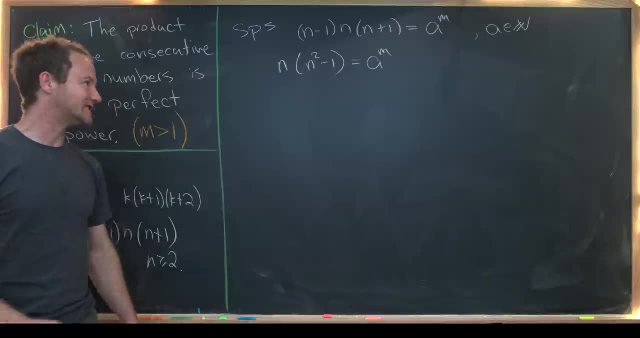 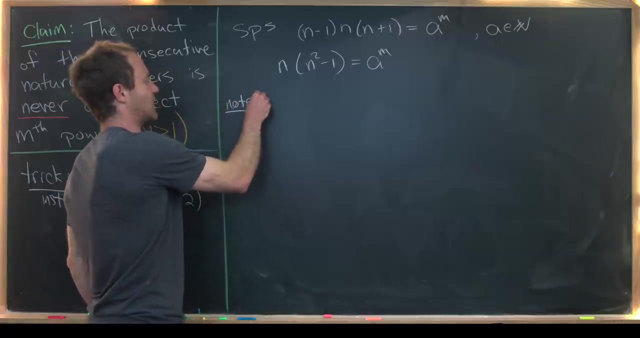 let's see where we can go from there. Now we can write this as n times n squared minus 1 equals a to the m. But now I want to look at the GCD of these two portions of the product. So let's maybe notice we have the following fact: We 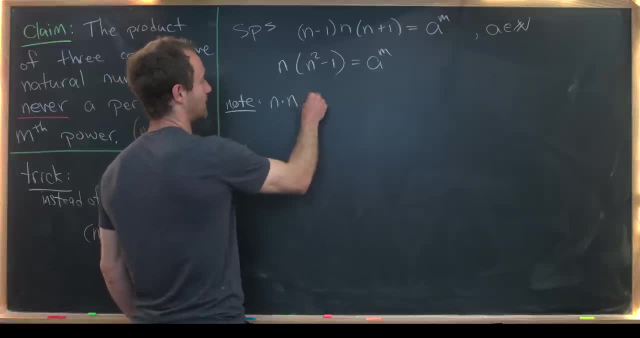 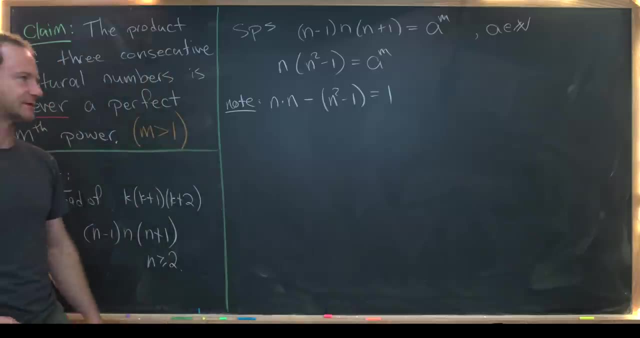 have n times n minus n, squared minus 1 is equal to 1.. So that's kind of an obvious formula. but what did we do? We wrote n, We took n and n squared minus 1, and then we found a linear combination of them that is equal to 1.. 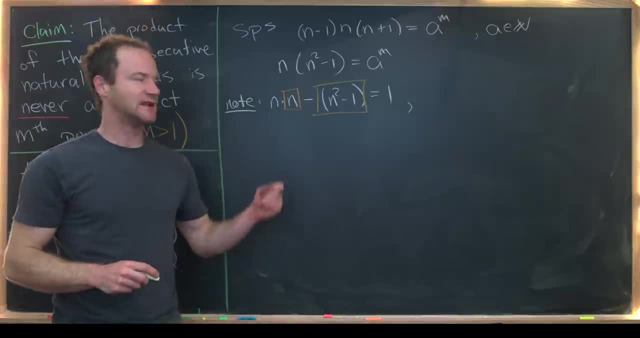 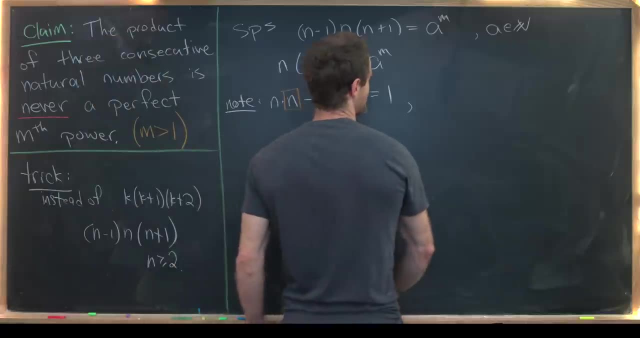 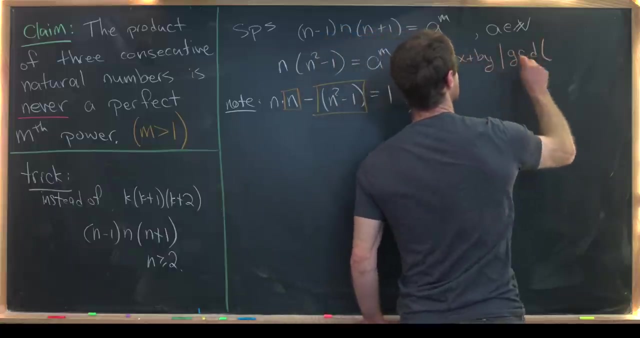 But now let's recall that that means that 1 divides the GCD of these two, these two things in these boxes. well, let's maybe spell that out up here: ax plus by always divides the gcd of a and b, where a and b are any integers and x and y are any integers. 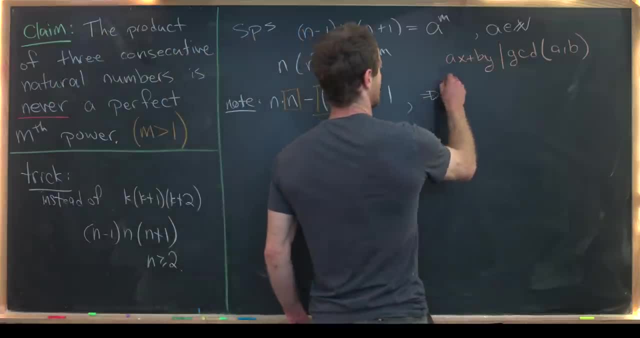 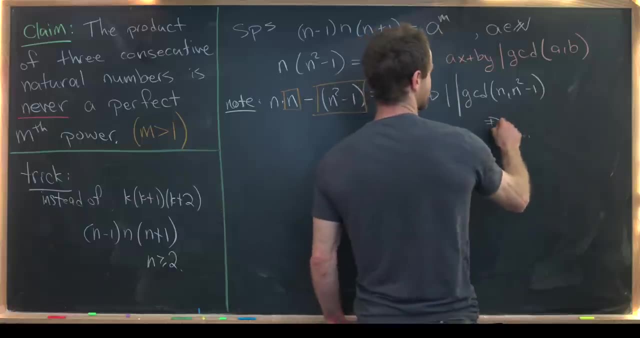 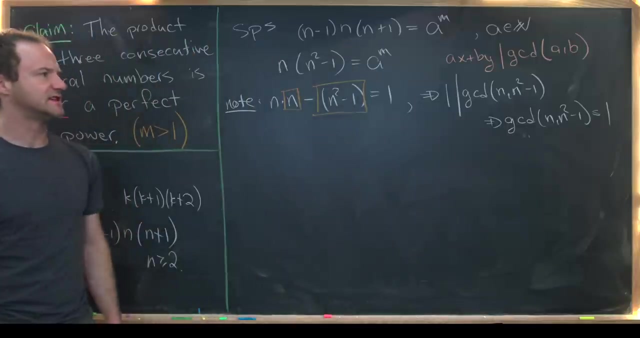 but that's exactly the kind of setup we have here. so that means 1 divides the gcd of n and n squared minus 1, which further tells us that the gcd of these two numbers is equal to 1.. great, but if the gcd of those two numbers is equal to 1 and their product is a perfect 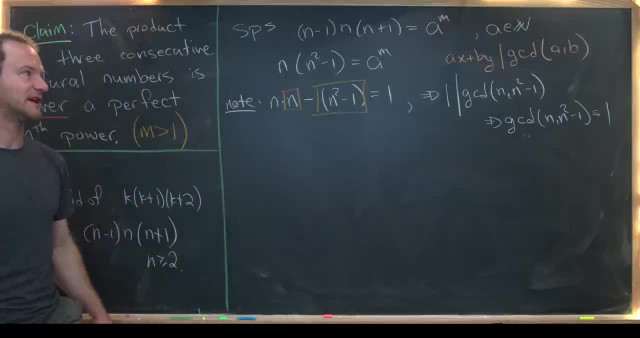 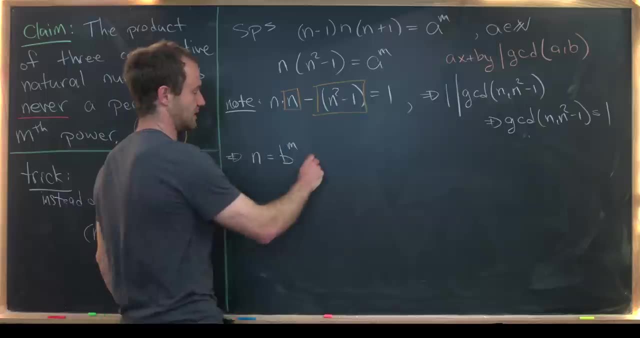 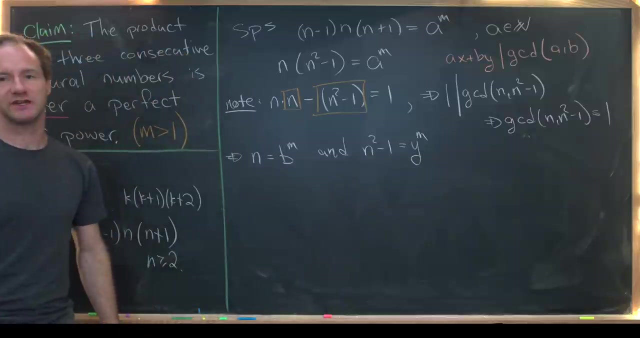 nth power. that means each one must be a perfect nth power in its own right. so we can write that down. now we have: n is equal to b to the n and n squared minus 1 is equal to y to the m. i'm going to use slightly different notation there now. i'll take this and square: 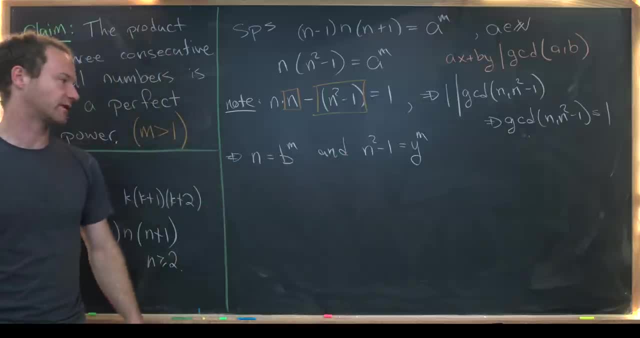 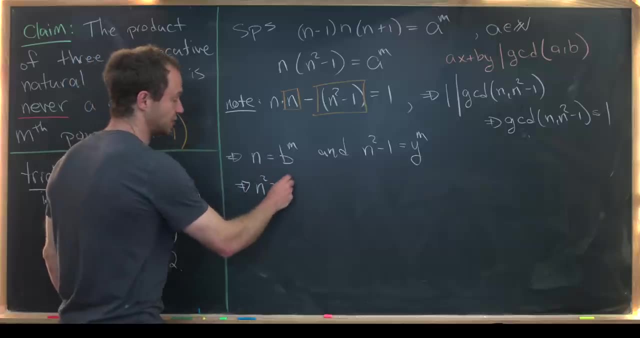 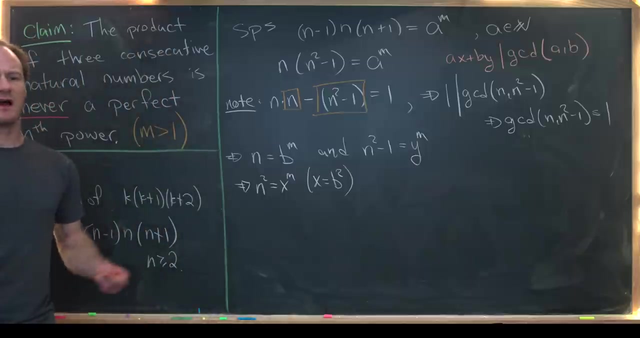 it because we've got n squared minus 1. we probably don't want to work with n, we want to work with n squared. so that's going to tell us that n squared is equal to b to the 2m, but i'm going to write that as x to the m, where x is equal to b squared. now i'm going to write: 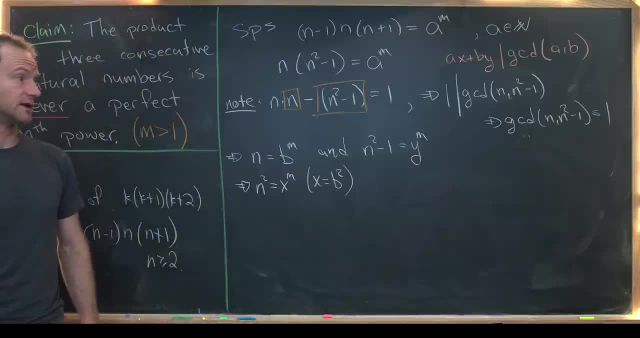 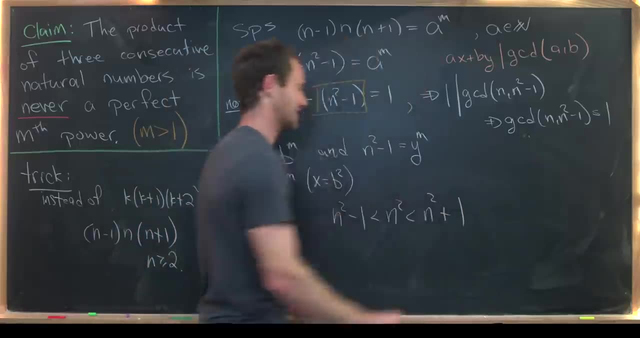 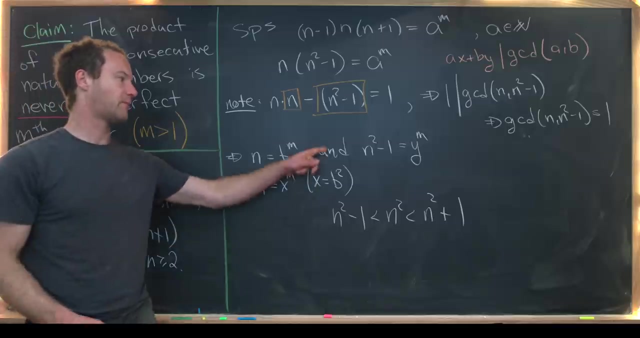 down what is maybe a very obvious inequality, and that's: n squared minus 1 is strictly less than n squared, which is strictly less than n squared plus 1.. so, like i said, that's a very obvious inequality. but now i'll take that inequality and rewrite it with parts from: